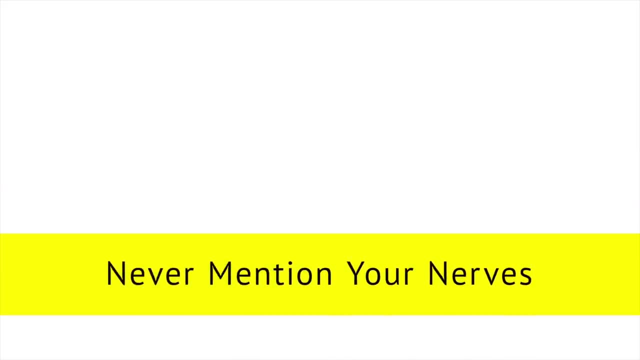 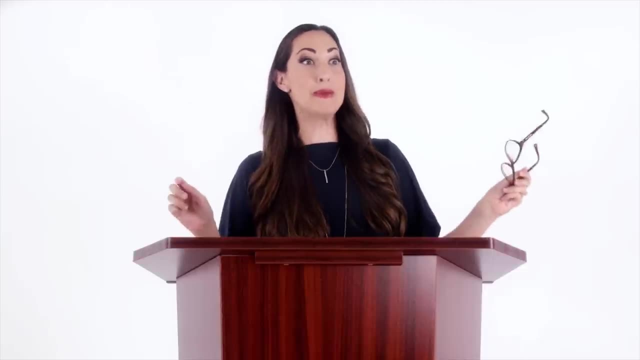 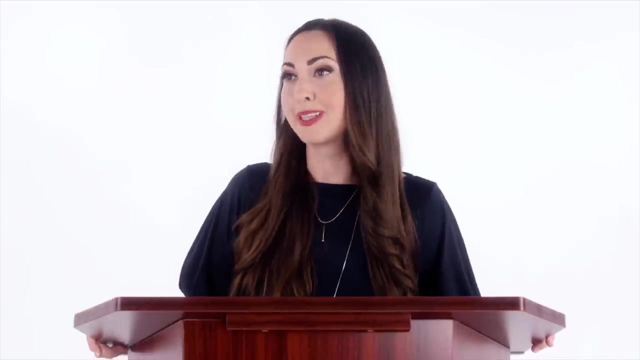 will think about. Never mention your nervousness. Do I look as nervous as I feel? Wow, there are so many people here, So I should start by saying that I am not a great public speaker, so this should be short. Many people think it's vulnerable or honest to start with. 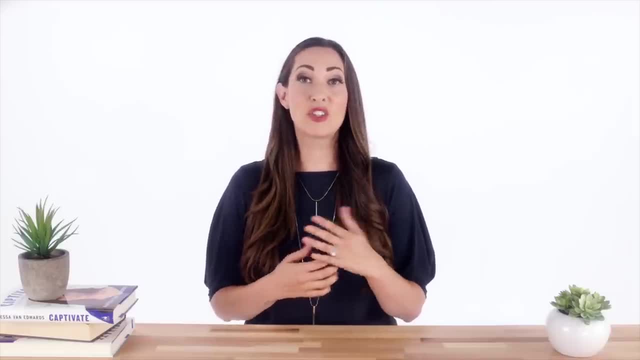 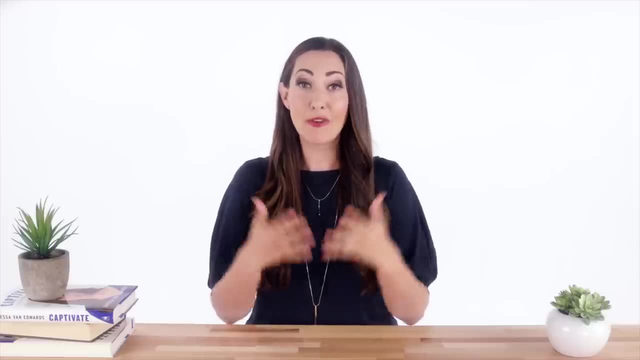 how nervous they are. But actually for your audience it's distracting. Why? Because the moment you mention your nerves, you make your audience nervous and they will begin looking for all the signs of your nervousness. It becomes a giant nerve-wracking wave that. 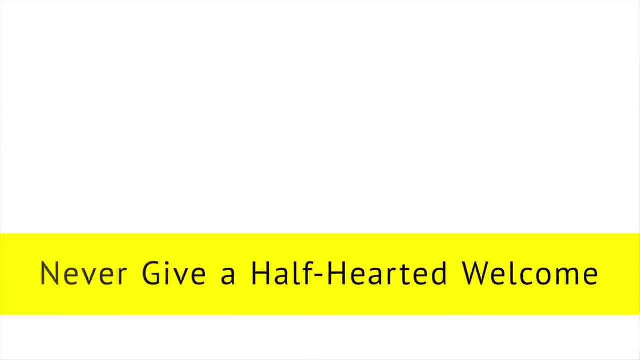 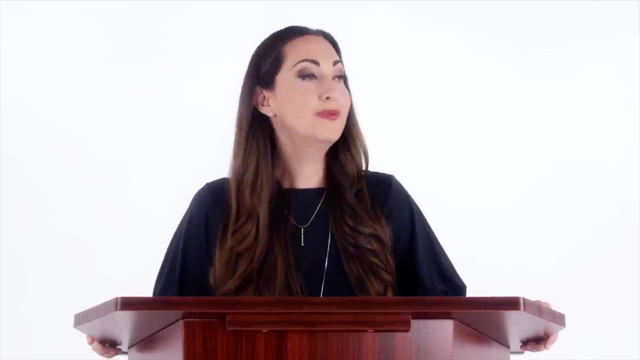 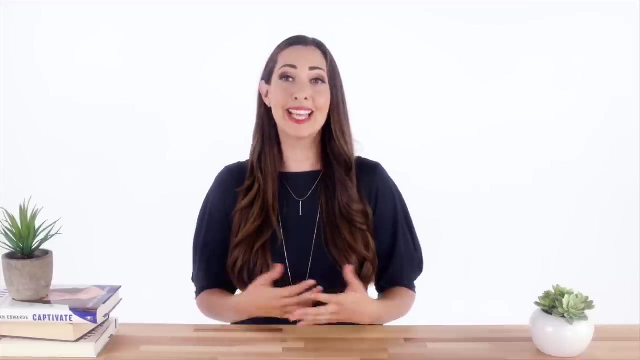 you start from stage Never give a half-hearted welcome. Thanks for having me. Well, it's so nice to be here. Thanks for that intro. Do not start with a boring nicety Or worse, saying something nice but not sounding like. 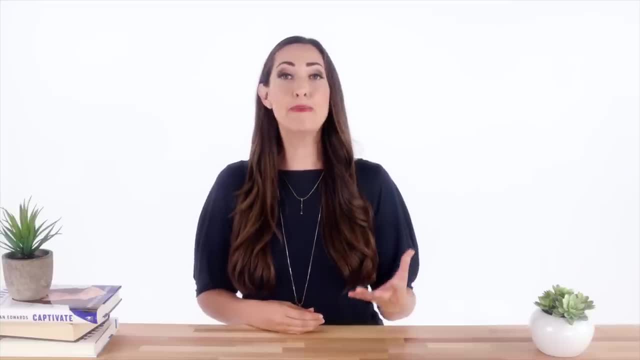 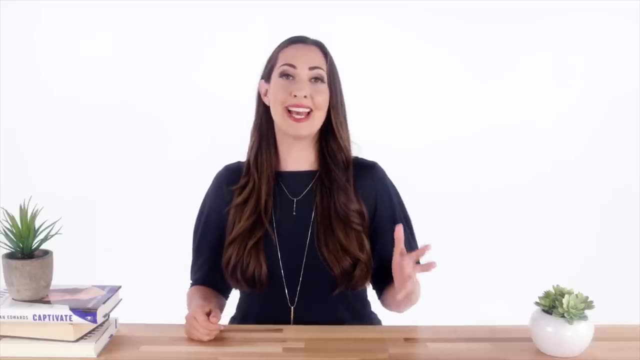 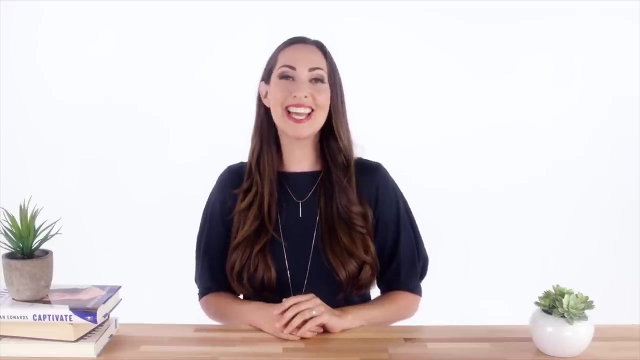 you mean it. I can't tell you how many times I have seen people get on stage and say I'm so happy to be here, but look so incredibly unhappy, as they say it Fake, fake, fake. The only exception to this is if you can turn it into a joke, like the amazing Ken Robinson. 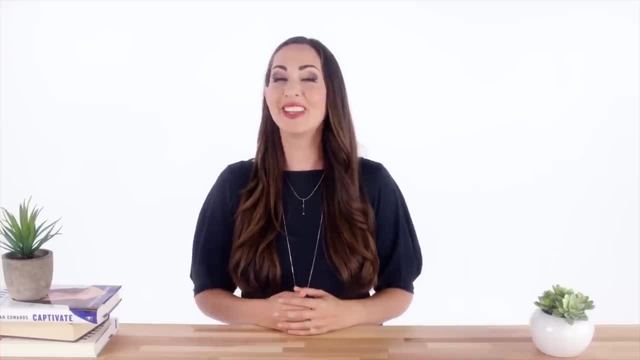 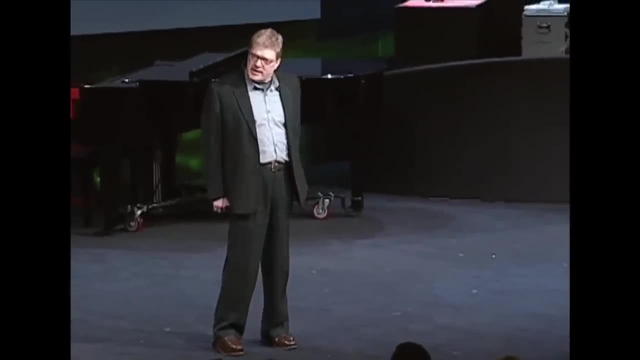 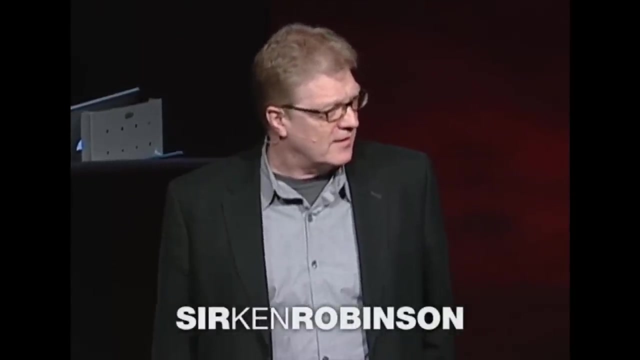 He opened his talk with a boring nicety, but then made it funny. Let's watch. Good morning, How are you? It's been great, hasn't it? It's been. I've been blown away by the whole thing. In fact, I'm leaving. 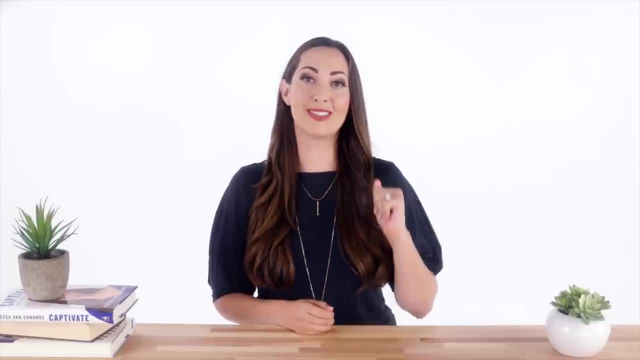 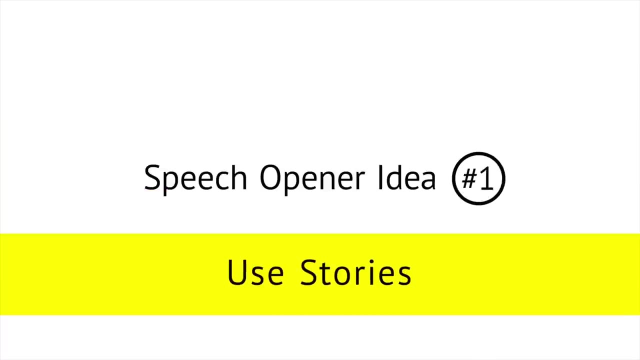 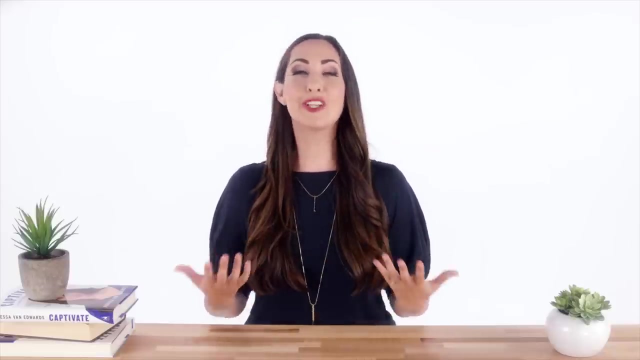 Okay, now that we've talked about the worst ways to start a speech, let's talk about the best Speech opener. idea number one: Use stories. The absolute best way to start a presentation is with a story. There is nothing better to capture the imagination and attention of an audience. Let's watch how David Brooks hooks. 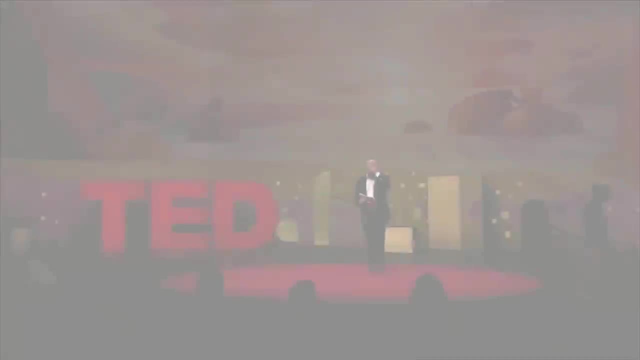 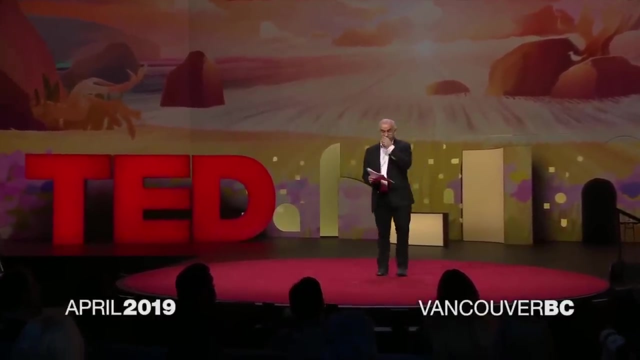 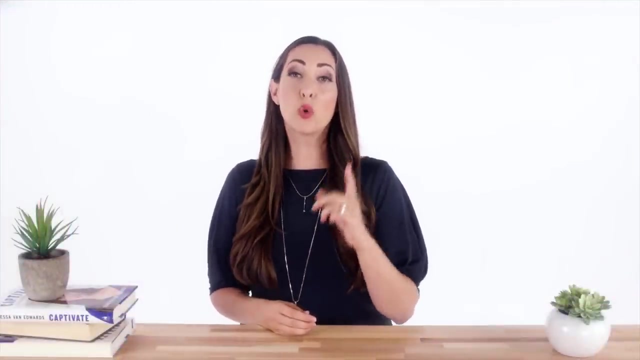 you in right now, Right at the start with his story. So we all have bad seasons in life And I had one in 2013.. My marriage had just ended and I was humiliated by that failed commitment. Whew Hooks you in right away. He gets right to the heart of it. Stories help your audience. 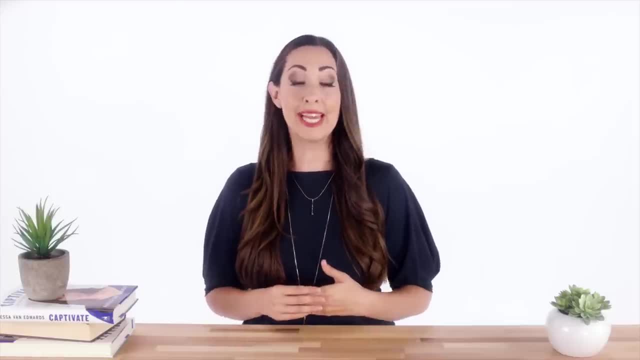 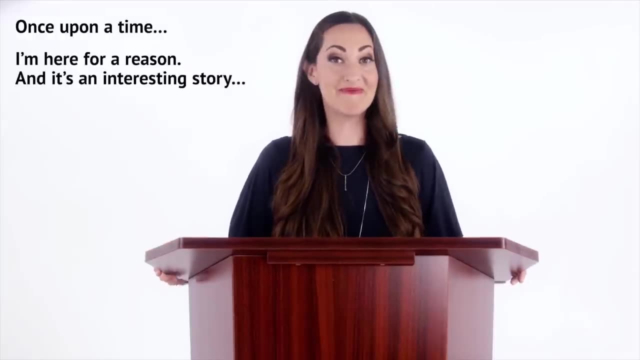 feel right there with you. Here are some fill in the blanks you can use to start your next speech with a story. Once upon a time, I'm here for a reason, And it's an interesting story. The best thing that ever happened to me was…. 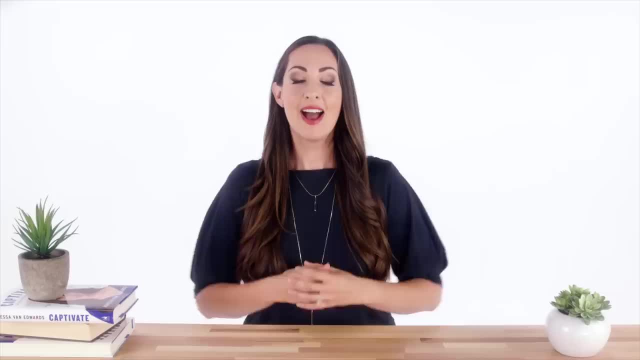 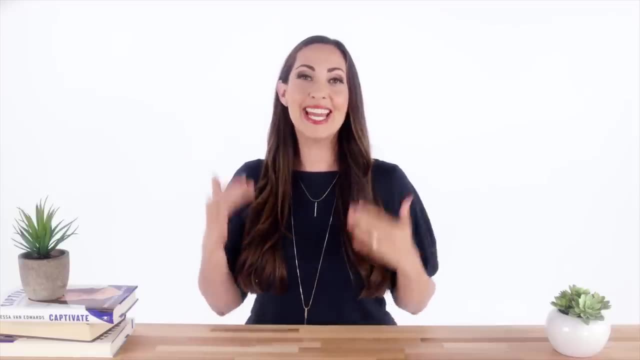 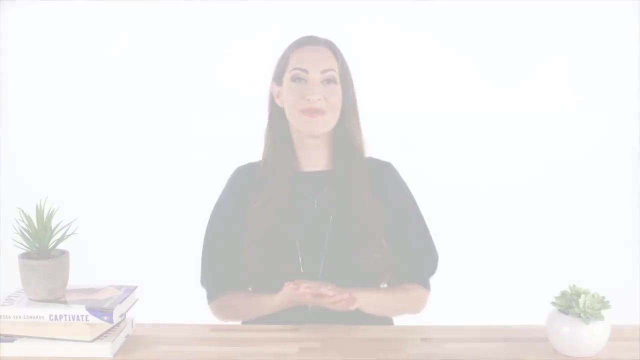 Speech opener. idea number two: Your big idea. I love when speakers share their big idea right up front. They don't make you wait for it, They dive right in. Let's watch how Stacey Smith starts off her talk with her big idea, framed in an interesting way. 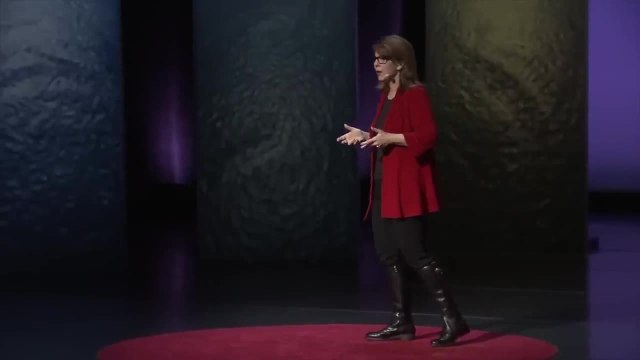 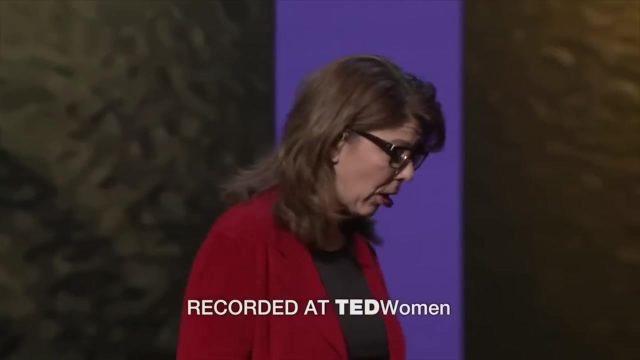 Today I want to tell you about a pressing social issue Now. it's not nuclear arms, It's not immigration, It's not the US Department of Defense, It's not the US Immigration And it's not malaria. I'm here to talk about movies. 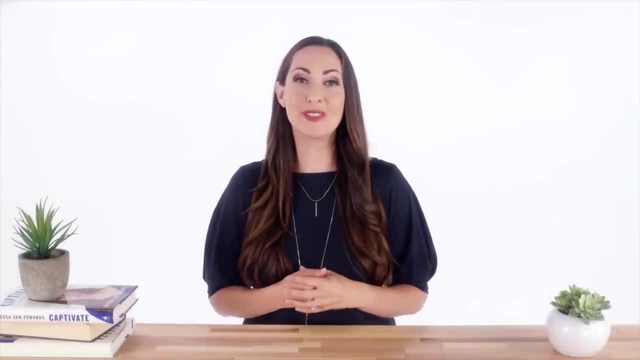 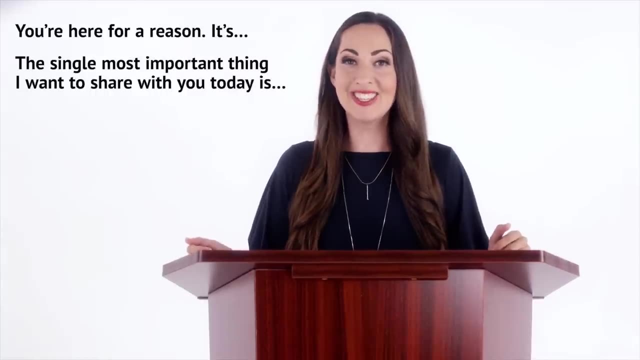 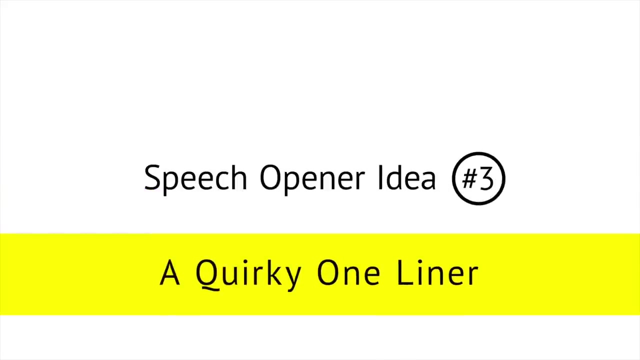 Here's some fill in the blanks you can use to open your speech. You're here for a reason. It's… The single most important thing I want to share with you today is…. Today I want to share a big idea. Speech opener number three: A quirky one liner. 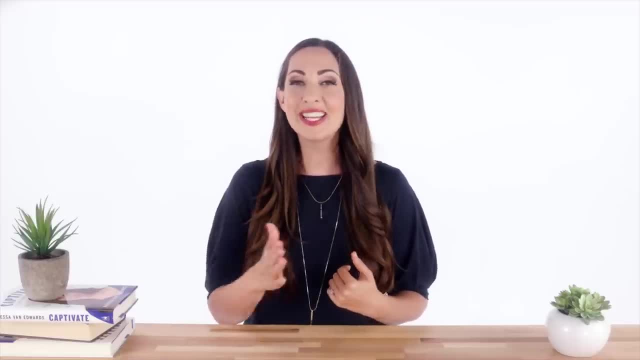 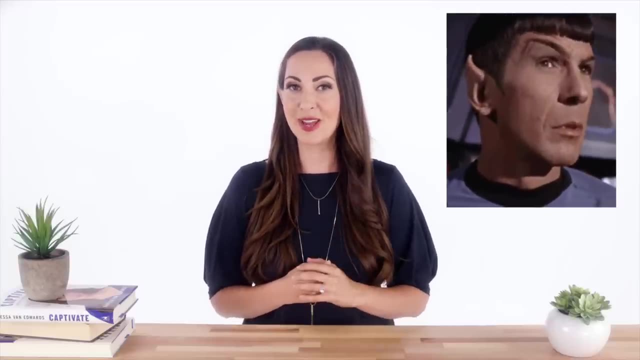 No one loves humor more than me, And I can promise you that your audience will as well, If you dare try to open your speech with something intriguing, Very intriguing. Humor or curiosity is a great way to start a speech on a high 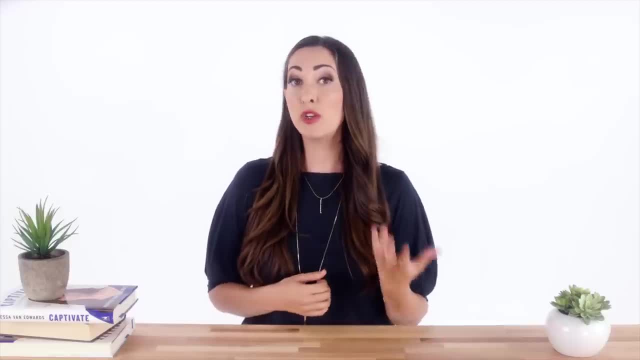 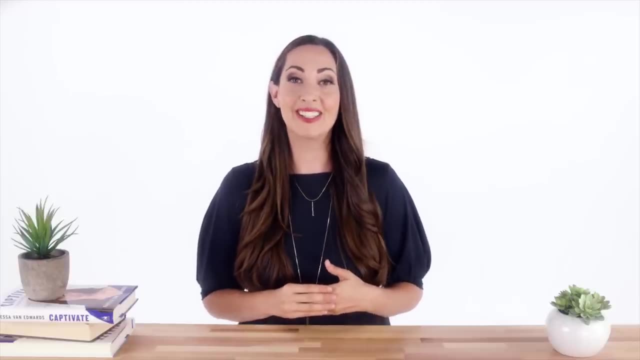 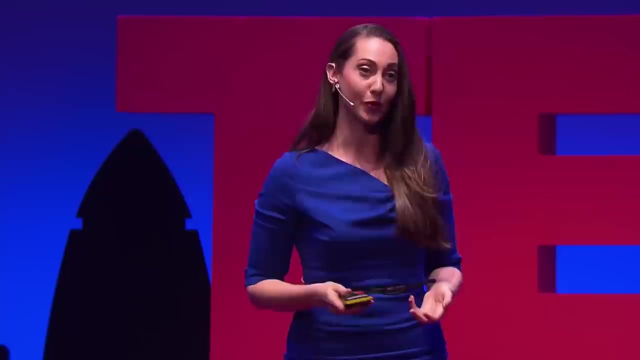 And please get creative. Think of an interesting fact about you, your audience or your topic that can lead you into your content. For example, when I gave my TED talk in London, I opened with my quirky one liner: Hello, My name is Vanessa and I am a recovering awkward person. 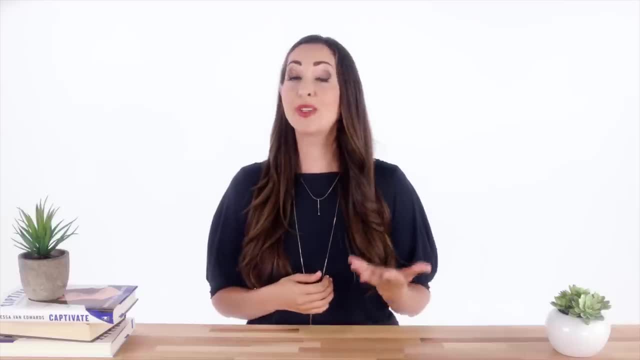 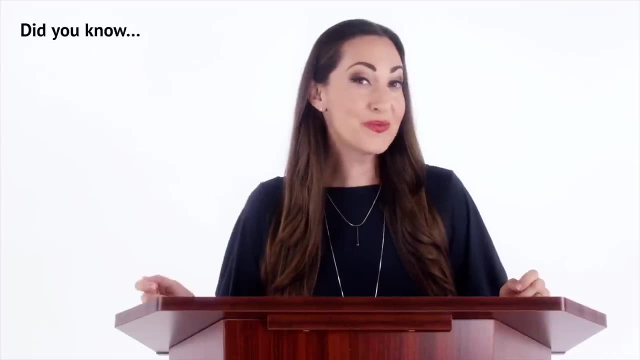 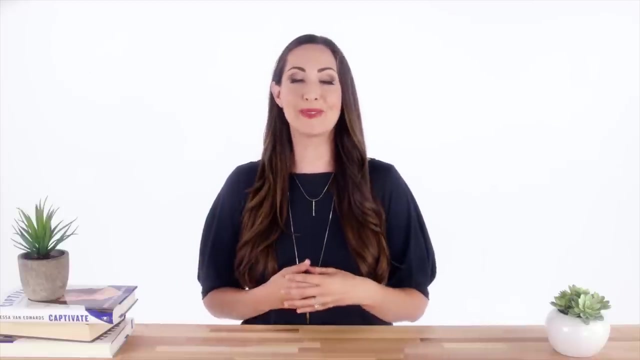 You can also use an interesting fact or even a question to the audience. Try some of these. fill in the blanks: Did you know… Do you ever worry about… Have you ever wondered…? For example, I do tons of corporate workshops and trainings, And here are some interesting. 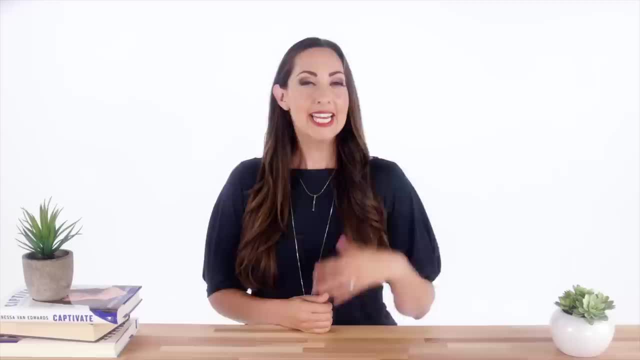 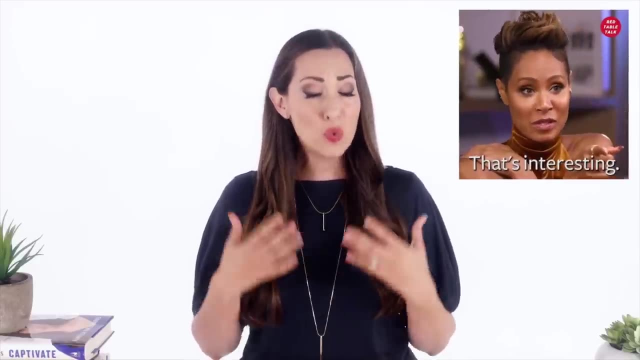 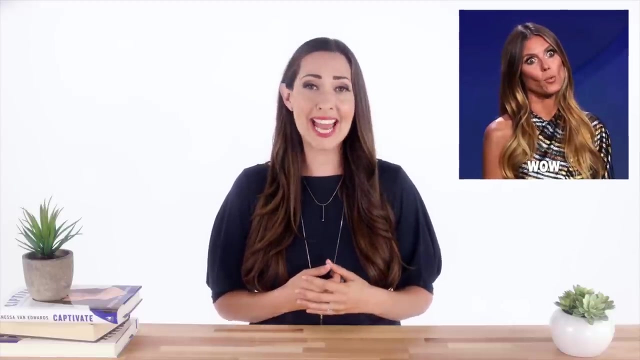 factoids. I start with that. hook the audience in. Did you know that it takes less than a second to make a first impression? Did you know that your non-verbal communication is… Is 12.5 times more powerful than your words? Did you know that we are lied to 200 times a day?